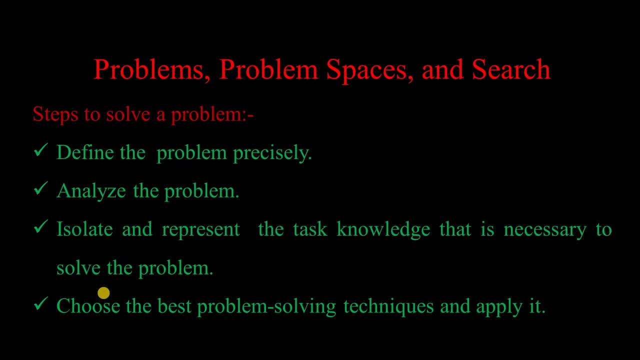 what we say, appropriateness of a various possible techniques for solving the problem. So we have to analyze the problem very, very importantly, and we have to identify which all features are more relevant to solve this problem. So when we are playing chess, what we are doing, we are just checking out what are the rules, We are just checking out what are the final conditions to win this game. So we are just tracking the rules which are to be orderly used for winning this game. 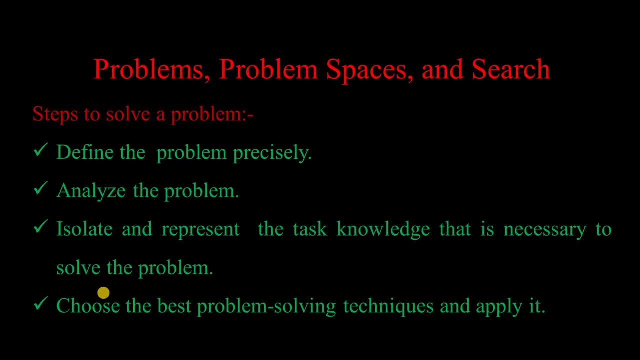 So analyze the problem. And the third step is: isolate and represent the task knowledge that is necessary to solve the problem. So important data type of abstraction is to be applied. And as a fourth step we can say: choose the best problem solving technique. That means there can be many different rules that can be applied at a single instance. So we have to choose the best rule which will lead to a low cost, or what we say more. 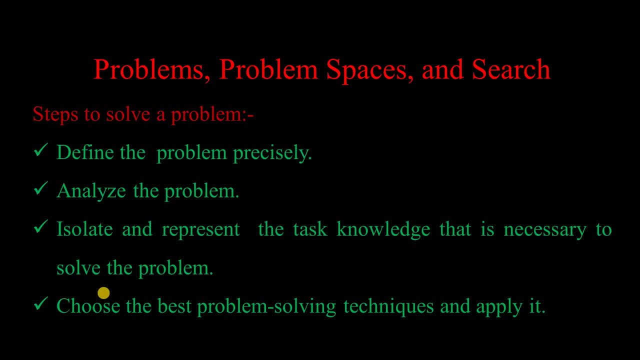 appropriate result. So we have to pick from that. So while playing chess in the first situation, starting from the initial state, we can have what we say- many different rules From that. we have to pick one to win the game. So what we will do is we have to pick one among the existing rules so that we will win the game. So we have to consider these points in mind. 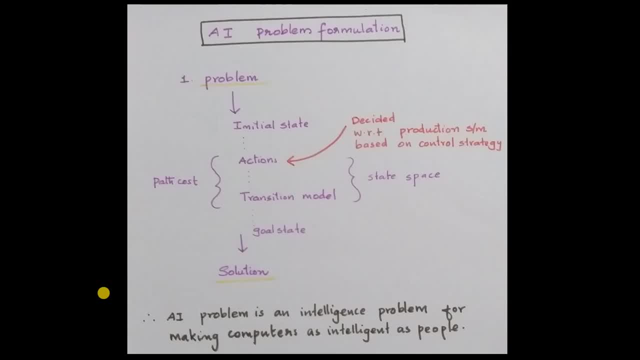 And moving on to the next, I have just briefed this particular definition in just like a flow chart. If you are considering an AI problem, we can define an AI problem formulation like this: There is a problem and we are starting from an initial state and we are traveling from the initial state to the goal state and in between we have several different actions, And this actions are decided with respect to the production system. What is production system? 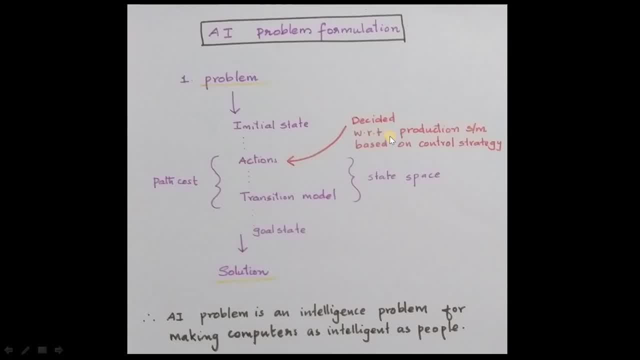 It's a set of rules and the production system from the production system. this actions are to be taken based on the control strategy. Control strategy means the dependency That means if two players, A and B, are playing chess, A's movement is decided with respect to that of B and B is playing with respect to the movement of A. Not a predefined action is being taking place. It is subtle dynamic. Their decisions are being changing dynamically. 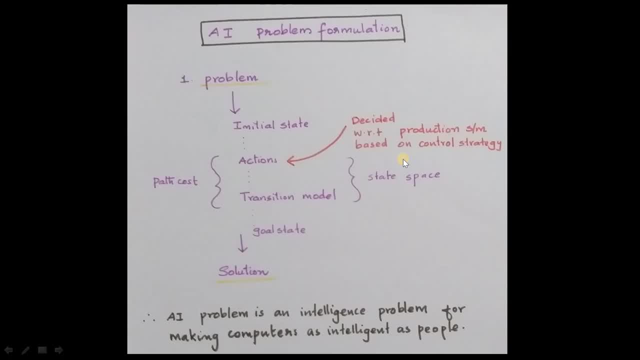 Because A want to win and the same go for B, So they both will take their own strategy so that they can win or they can defeat the other one. Okay, So these are the production system and control strategies and several transition is being taken place here and in this state space. we are getting a transition model and traveling from an initial state to the goal state. there are different, different states, And if the state is similar to the goal state, then we are going to have a transition model. 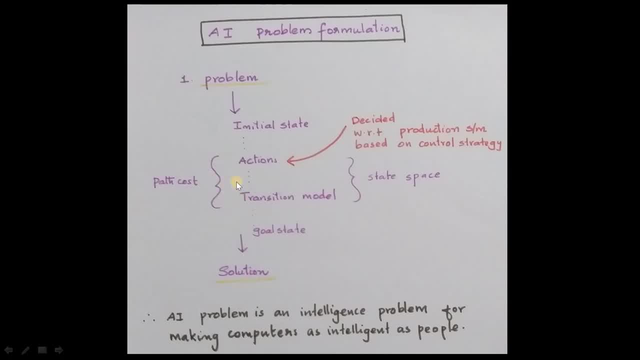 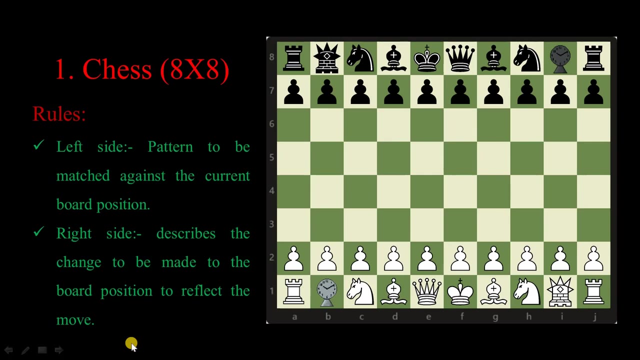 We will get the solution, and the entire cost of these traversing is called the path cost. Therefore, an AI problem is an intelligence question or a problem for making computers as intelligent as people And for defining or for explaining how a problem is being formulated or how a problem is being represented. we are using the example of chess, So we have in front 8 into 8.. 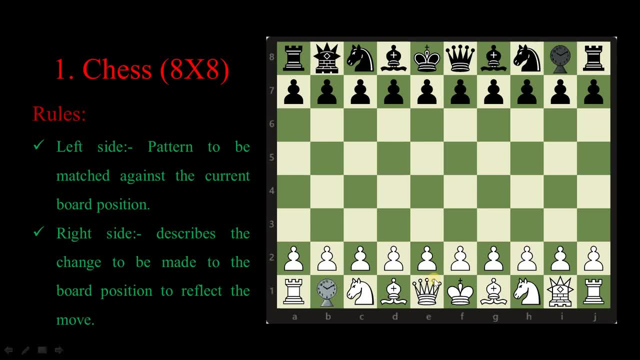 Chess board. This is not actually an 8 into 8 chess board. This is having more than 8 columns here. We have 8 rows here And if we check, we have 2,, 4,, 6, 8 and 10 columns here And we can, we are- expressing the results in by using an 8 into 8 chess board. I have just given an image so that you will rewind your memories in your memory. 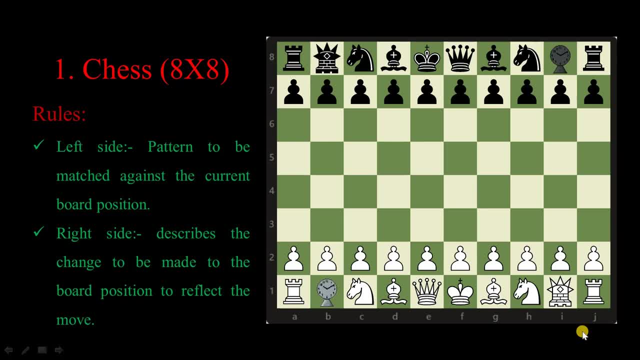 In playing chess. Okay. So if we are thinking, just suppose we start with a problem statement that is play chess. So, although we are, there are a lot of people whom with we can play chess, But making a program, Okay, Making a program or building a program that could play chess, This is very, very what we say, interesting task. So this board position, we can take it as a what we say. 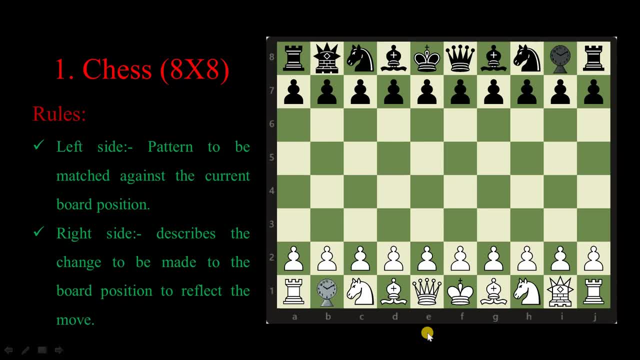 Initial state And in the final state we have the king of anyone defeated. That's according to a war. I have said it. So while programming this, we have to first decide an algorithm for this and for writing the algorithm. we should have the rules here. So how to mention the rules while playing the chess in the viewpoint of a player, And in the viewpoint of a human, as well as in the viewpoint of a machine? 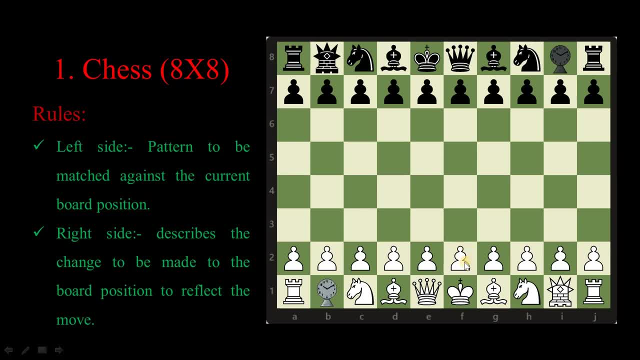 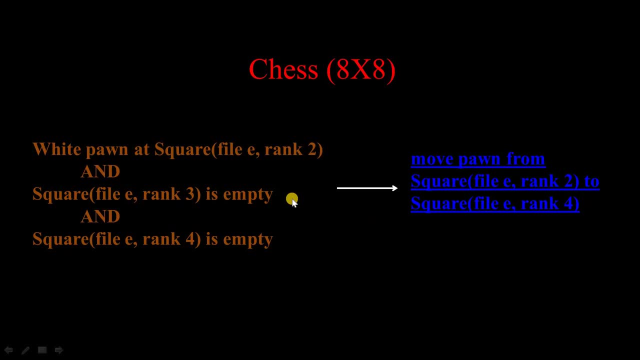 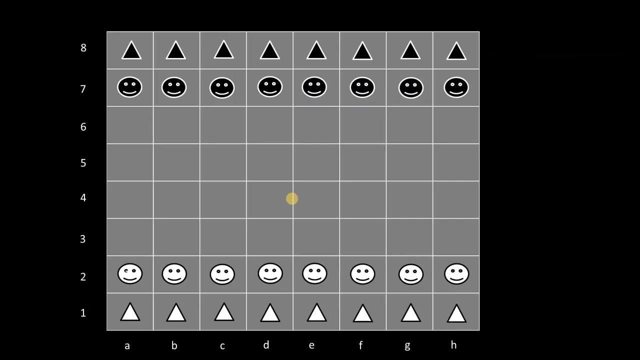 So think about this particular coin. So if the rule is we can move in two squares, Okay. So for moving this coin to two squares, or for moving this coin, we can say the rule like this: Okay. So I'll explain this rule by using a small demonstration. You just check this. So suppose this is my chess board And I am, for example, 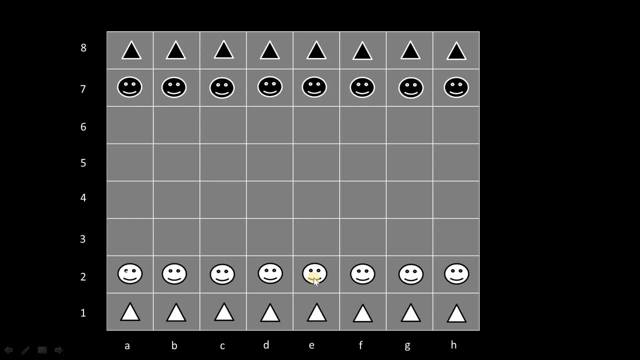 Focusing on this particular coin. I have to. I just I would like to move this coin forward. So what is the rule which will support moving this? Okay, So I'm making a rule or I'm considering the formulation of a problem. So, for moving this particular coin, What are the preconditions? The preconditions is that in this square there should be a coin. Okay, We should have a white pawn here, And this space or this cell should be empty. That means 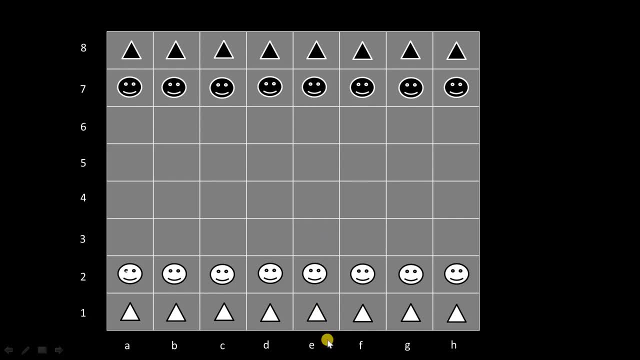 The, the cell in the column E, row three, And same is here. The cell in the column E, row four should be empty. So we can demonstrate it like this: We are considering these three cells for moving, So what can be the rules? We are writing the rules in the format of an if, then condition format. Okay, So if, what are the conditions to move? 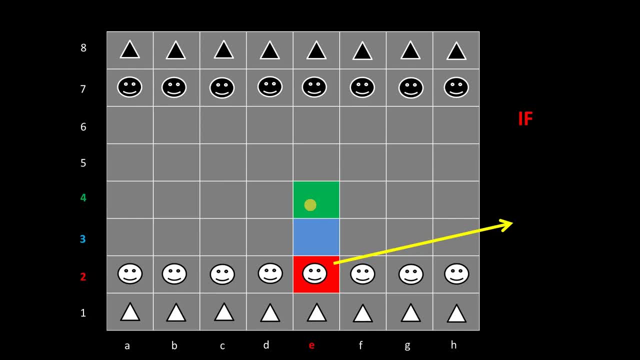 This particular coin. If the first consideration is that this square should contain a pawn And its color should be white, That is, a white pawn at square Which square? File E, rank two. File E, rank two. Okay, It's already there. And what's the next consideration? Next consideration is that Square File E rank three. That means this square should be empty. What's the next consideration? 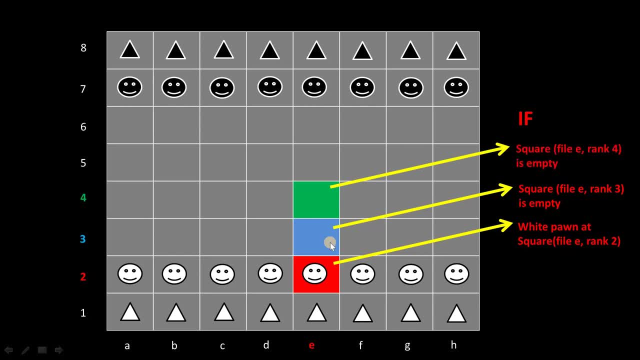 Square File E, rank four. Okay, It's also to be empty. And if all these three considerations are What we say, Okay, Then This is the if part, or the left part of the rule. And what is the right part? It is a then part. Then what happens? We are moving the pawn from the square E- Okay, File E, rank two, To the square File E, rank three. That means 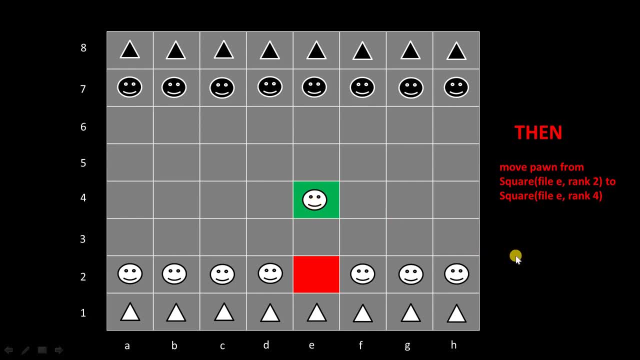 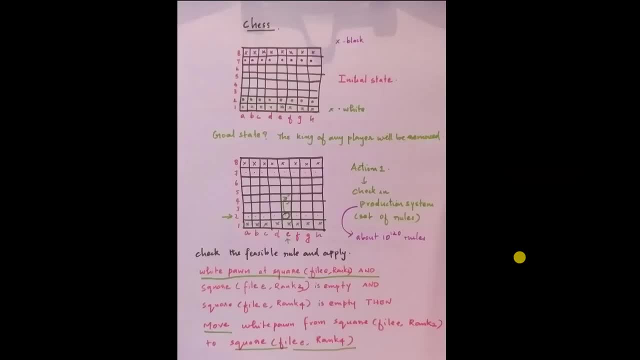 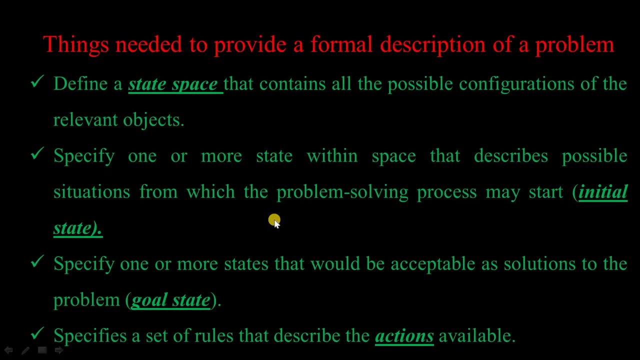 File E, rank four. So this is what we explain, How we explain the problem formulation with the example of chess. Okay, So I'm just given it in what we say, not format. You just go through this, Okay. So if we are formally describing the problem, We can define it in different terms. As the first, we have the state space. That means we have the production system, We have a space that contain all points. 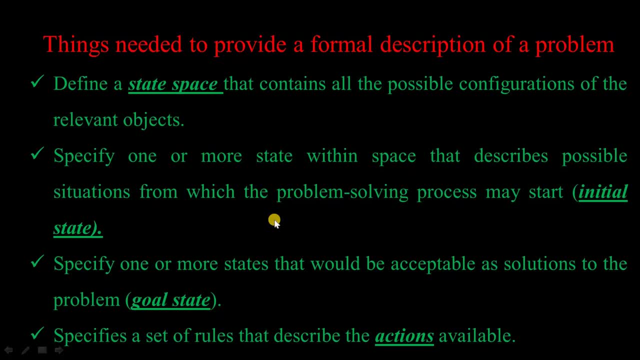 We have the possible configurations of the object, movements Or the play Or the game- Okay, And we have an initial state- That means the state with which the game starts, And we have the goal state. That means the final state. By achieving that particular state, The game ends. Okay, And the movement from one state to another is mentioned by using the term actions. Okay, And that's it. That's it all. 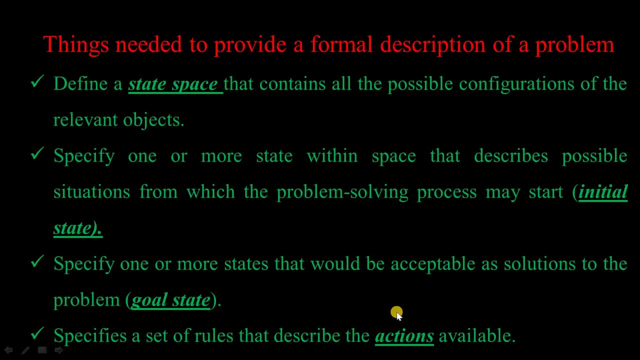 About what a problem in AI is And how a problem is formulated in AI And, of course, we have already described how a rule is being formed with respect to an example of playing chess. Okay,